Meet Anne. She often shops from wwwshoppingcartcom. She has her information, like email ID, address and credit card details, saved on the website to enable a faster and hassle-free shopping experience. The required information is stored in a server. One day, Anne received an email which stated her eligibility for a special discount voucher. 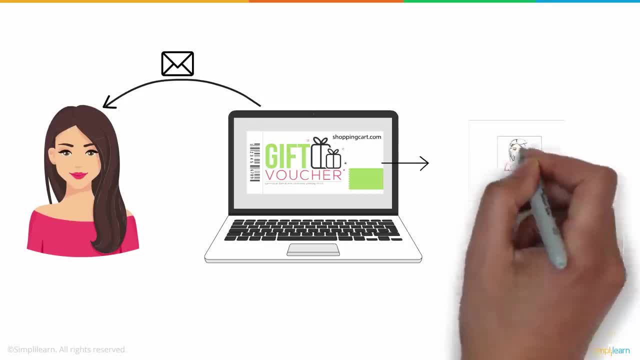 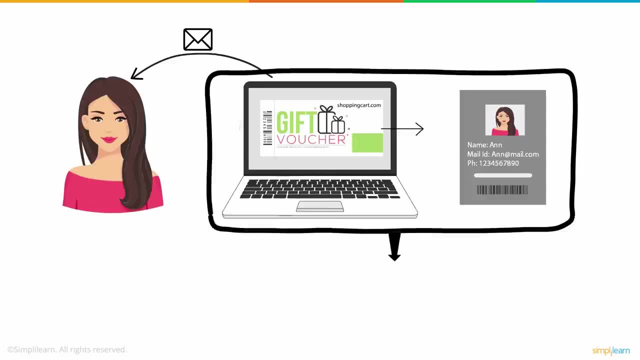 from shoppingcartcom. In order to receive the coupon code, she was asked to fill in her shoppingcartcom account credentials. This didn't seem fishy to her at the time, as she thought it was just an account verification step. Little did she realize the danger she would be facing. 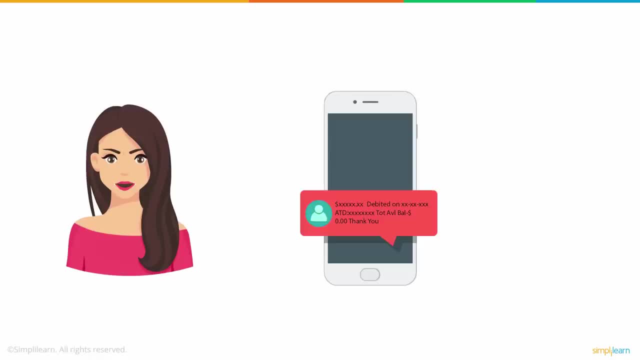 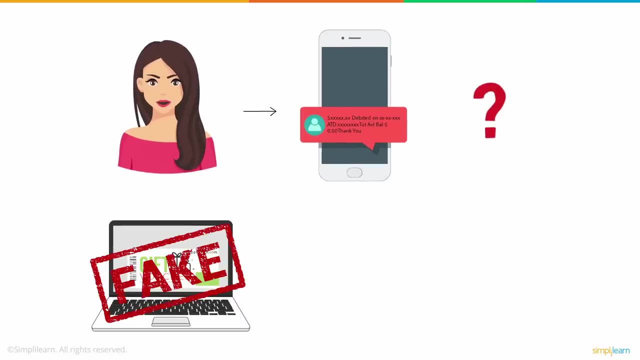 She was knocked off her feet when a substantial amount of money was wiped off her account. How do you think this happened? Well, yes, the email she received was fake. Anne's shoppingcartcom account was false, witnessed unauthorized access from a third party. 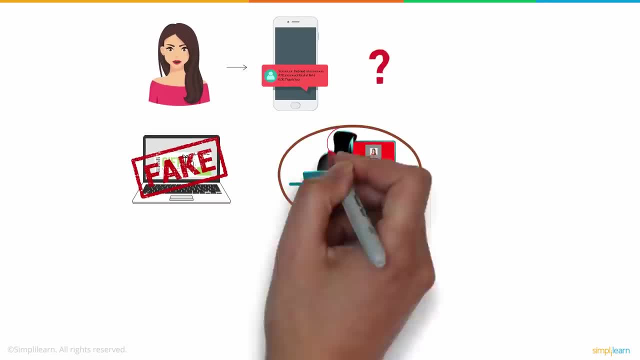 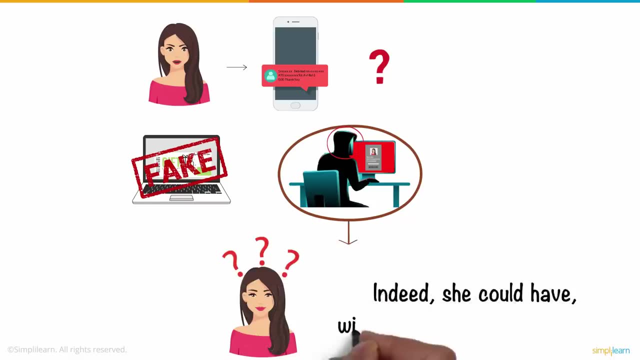 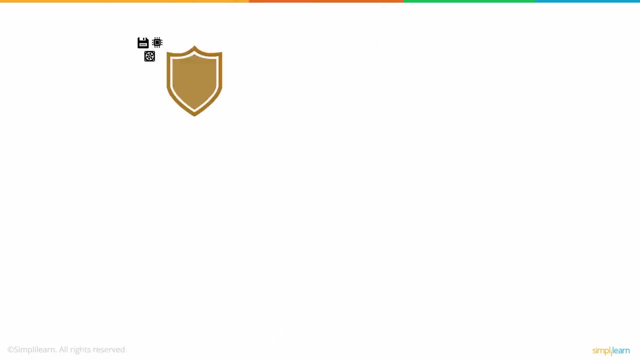 This type of attack is known as a cyber attack, and the person who carries it out is called a hacker. Could Anne have prevented this attack? Indeed, she could have with the help of cybersecurity. Cybersecurity involves techniques that help in securing various digital components. 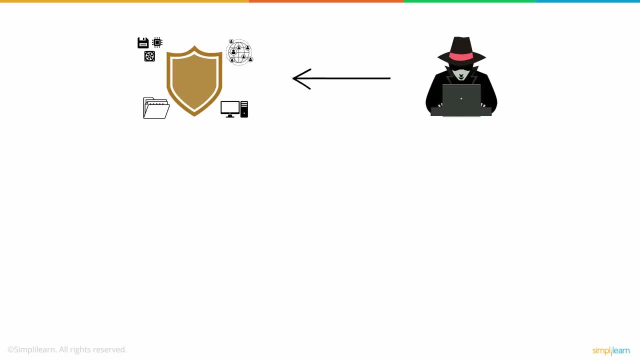 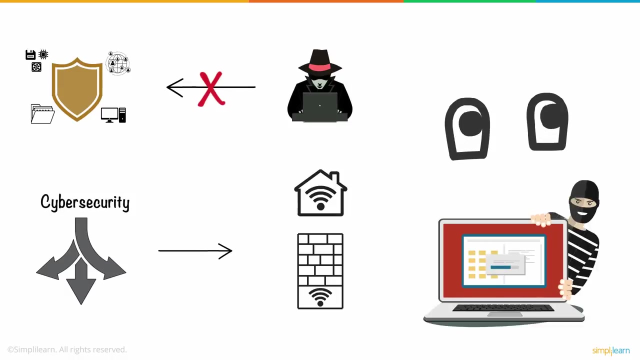 networks, data and computer systems from unauthorized digital access. There are multiple ways to implement cybersecurity, depending on the kind of network you are connected to and the type of cyber attacks you are prone to. So let's take a look at the various cyber attacks that Anne could have been exposed to. 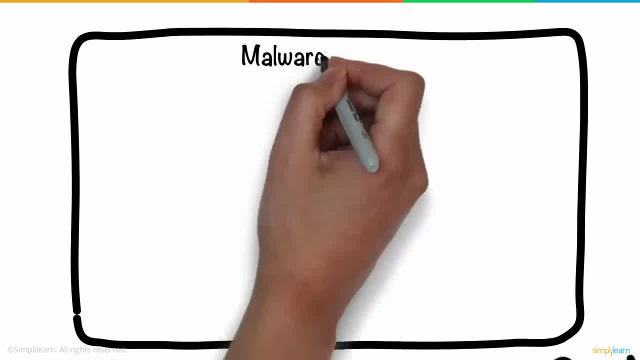 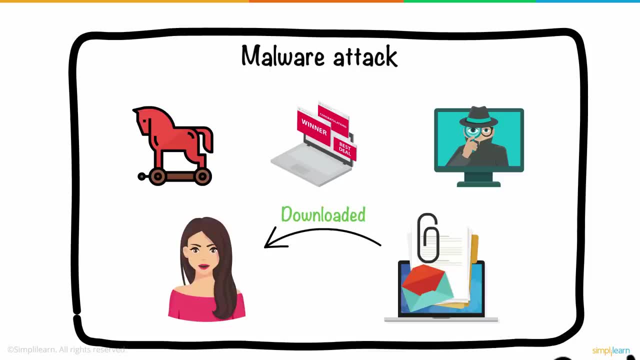 One of the most common types of cyber attacks is a malware attack like Trojan, Adware and Spyware, to name a few. Had Anne downloaded any suspicious attachments online, her system could have gotten corrupted by certain malicious viruses embedded within the attachments. 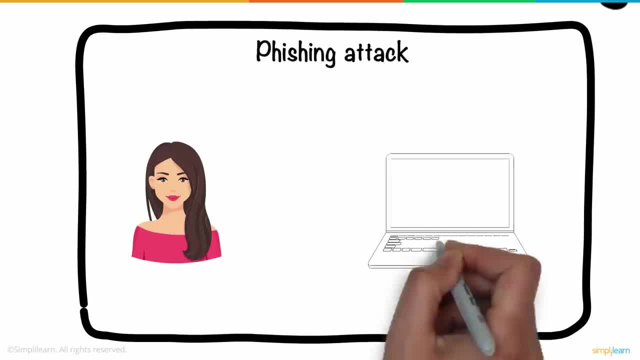 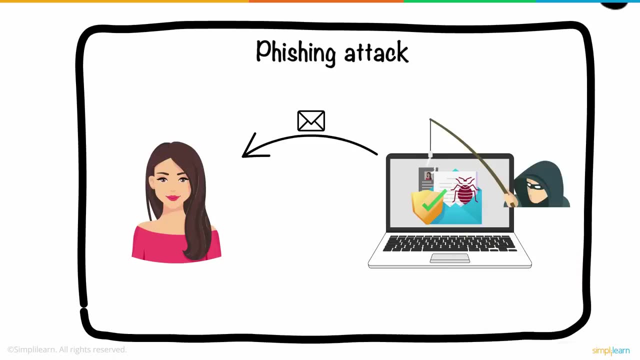 Next is cybersecurity. This is a phishing attack, the type of cyber attack which Anne experienced Here. the hacker usually sends fraudulent emails which appear to be coming from a legitimate source. This is done to install malware or to steal sensitive data like credit card information and login credentials. 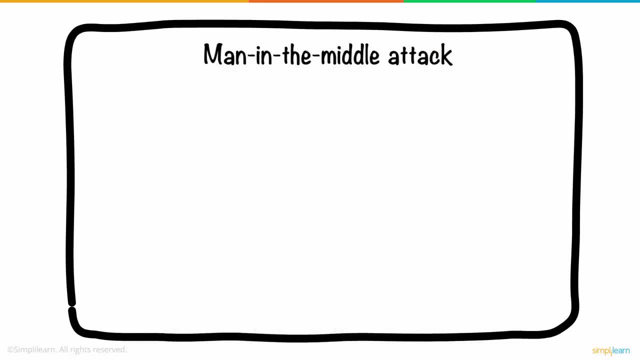 Another type of attack is the man-in-the-middle attack. Here the hacker gains access to the information path between Anne's device and the website's server. The hacker's computer takes over Anne's IP, takes over Anne's IP address. By doing so, the communication line between Anne and the website. 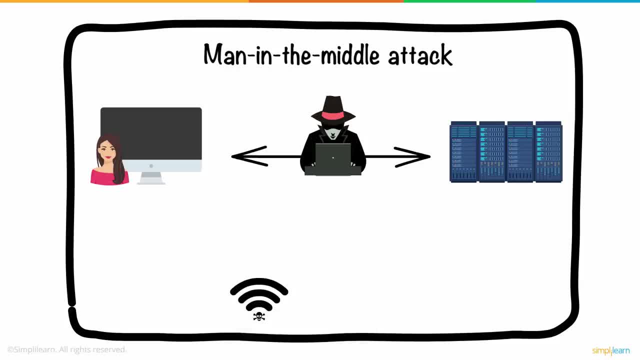 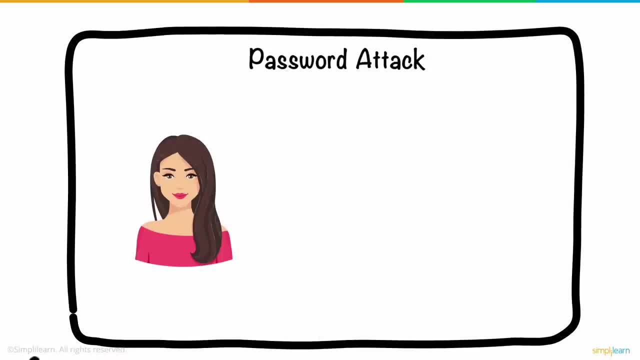 is secretly intercepted. This commonly happens with unsecured Wi-Fi networks and also through malware. Password attack is one of the easiest ways to hack a system. Here, Anne's password could have been cracked by using either common passwords or trying all possible alphabetical combinations. 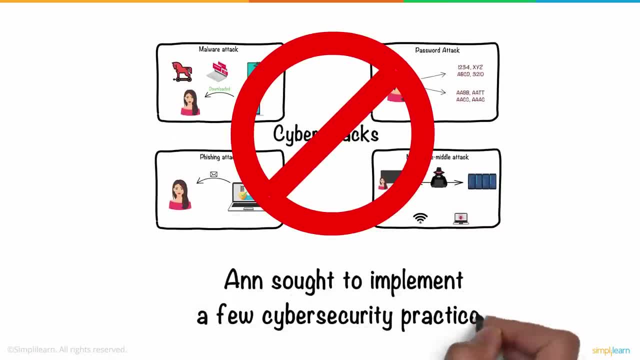 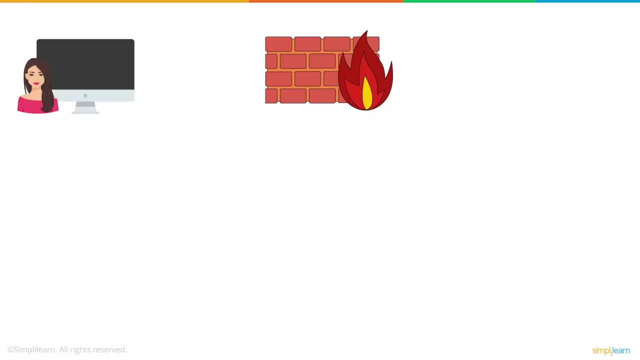 To prevent future cyber attacks, Anne sought to implement a few cybersecurity practices. First, she installed a firewall. As the name suggests, it is a virtual wall between Anne's computer and the Internet. Firewalls filter the incoming and outgoing traffic from your device to safeguard your network. 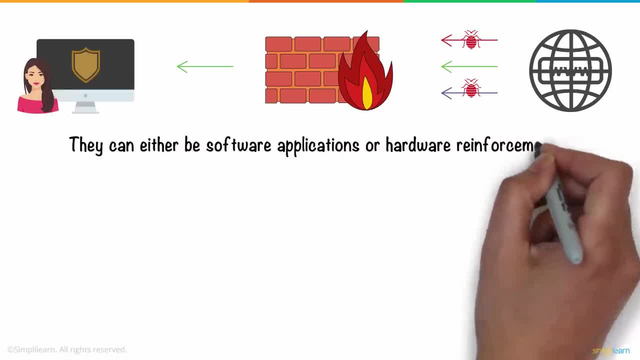 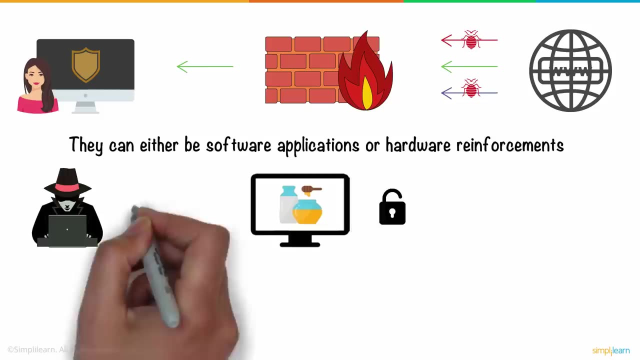 and they can either be software applications or hardware reinforcements. Secondly, Anne implemented honeypots. Just like how flowers attract bees, dummy computer systems called honeypots are used to attract attackers. These systems are made to look vulnerable in order to deceive attackers. 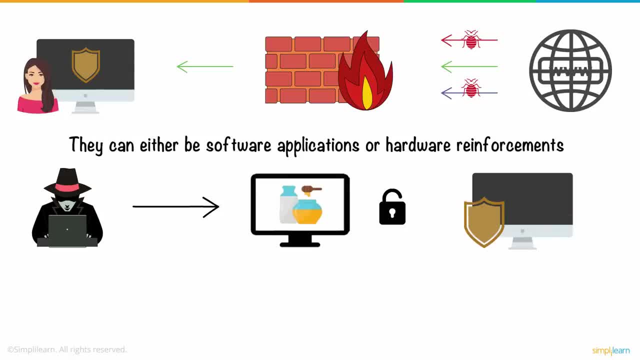 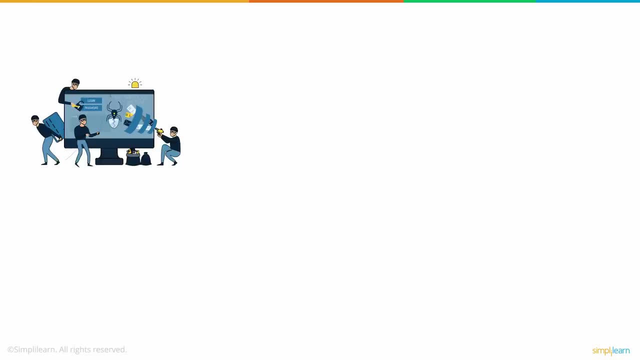 and this in turn defends the real system. In addition to these, she also decided to use unique alphanumeric passwords, antivirus software and started avoiding mails from unknown senders. That was Anne's story. Cyber attacks are not just confined to individuals. but also to public and private organizations. The cyber attacks carried out in such places are more deadly and they result in colossal losses. Motives of such attacks are many, starting from tampering with crucial data to monetary gains. Let's have a look at a few of the cyber attacks. 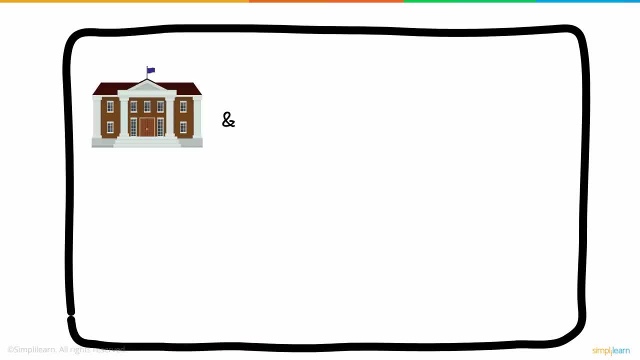 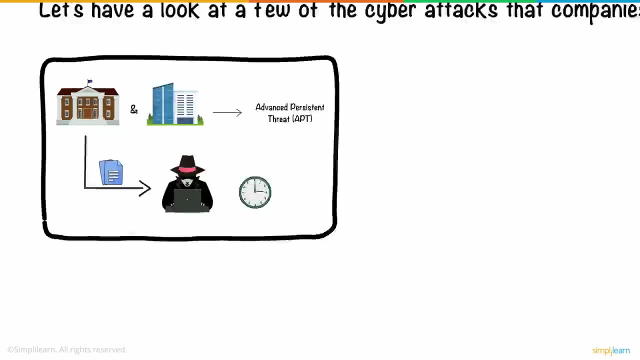 that companies are subjected to. Various public sector organizations and large corporations face the Advanced, Persistent Threat In this form of attack. hackers gain access to networks for a prolonged period in order to continuously gain confidential information. Companies also witness the Denial of Service attack. 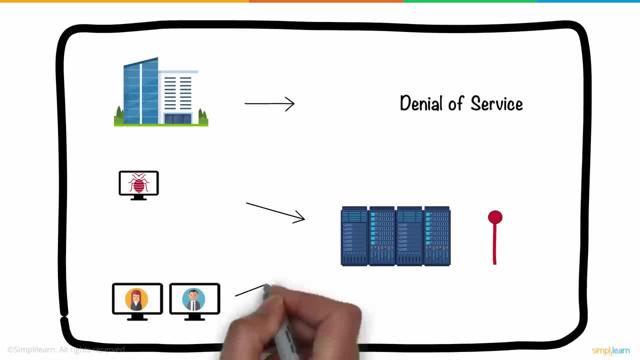 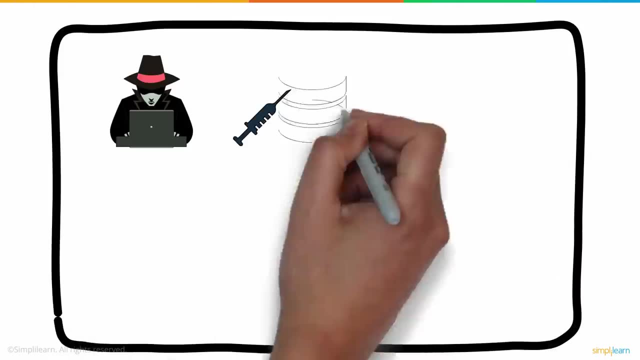 where networks are flooded with traffic, which in turn leaves legitimate service requests unattended. A variant of this is the Distributed Denial of Service attack, when multiple systems are used to launch the attack. When a hacker manipulates a standard SQL query in a database-driven website. 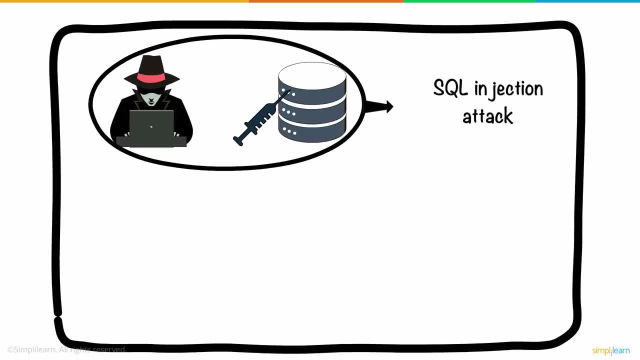 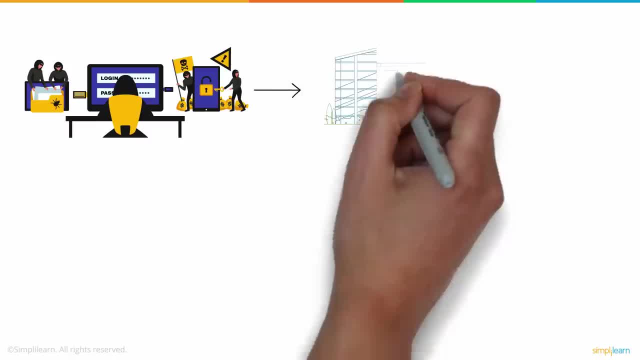 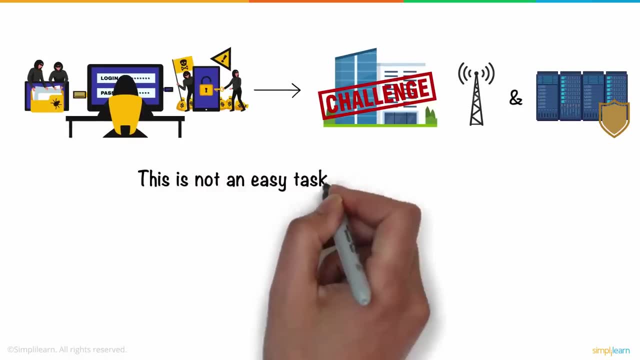 it is known as a SQL injection attack. By doing so, hackers can view, edit and delete tables from databases. Amidst a plethora of cyber attacks, it is indeed a challenge for organizations with several networks and servers to ensure complete security. This is not an easy task.